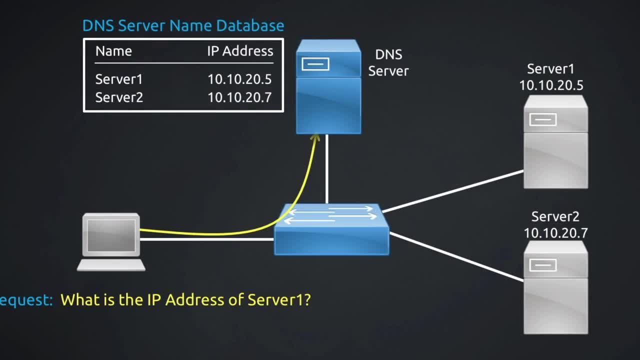 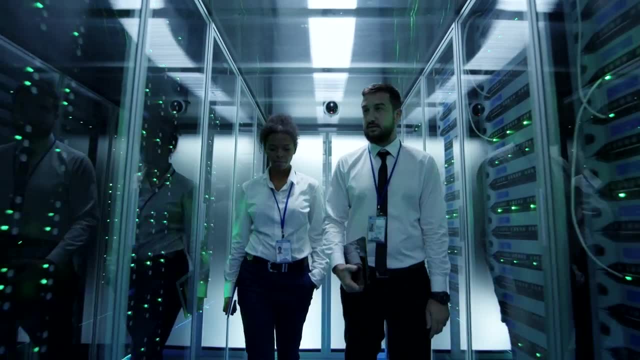 design as well. You get to create diagrams and map out. use creativity, map out different networks and use your creative mindset to do that. You also get to work with people. You get to present these things to people. You get to go, present solutions and also fix things for people. 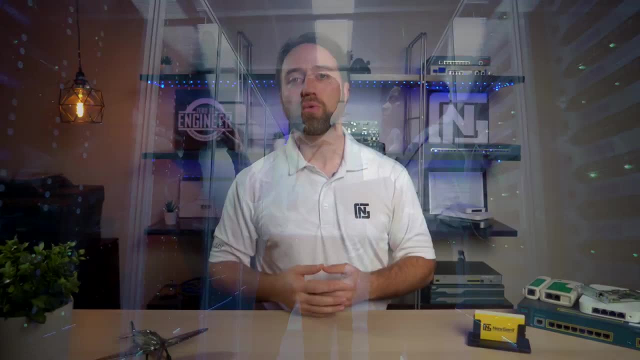 So there's very much a balance of technical things and working with people And for me that brings a lot of enjoyment to my day And I love actually going to work every day and working with people. And I love going to work every day and working with people. 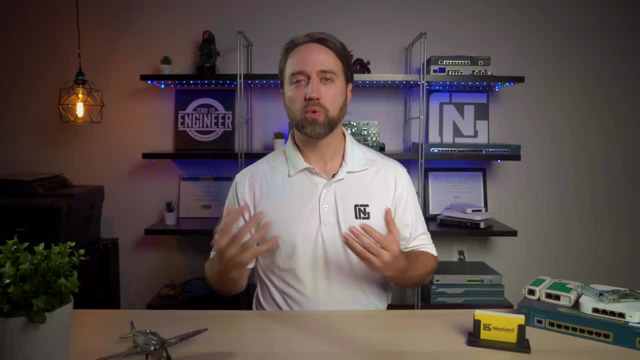 I love going to work every day as a network engineer because of these things. I love working with people and I love working with technology. Very much a good balance of that. So again, that's number one. The number one reason why I would recommend this career is the work. 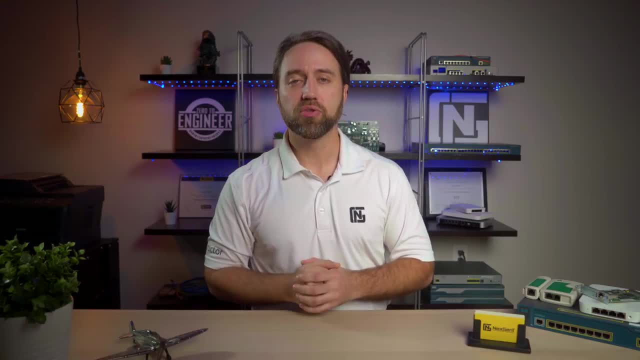 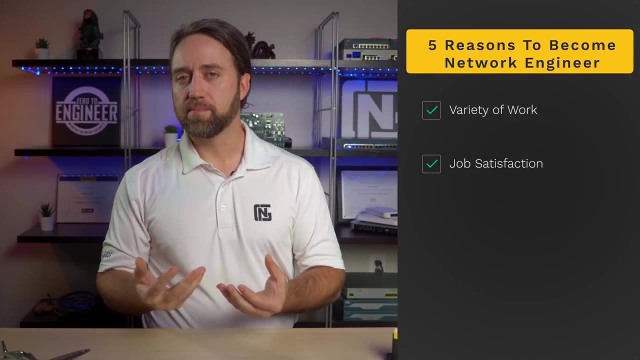 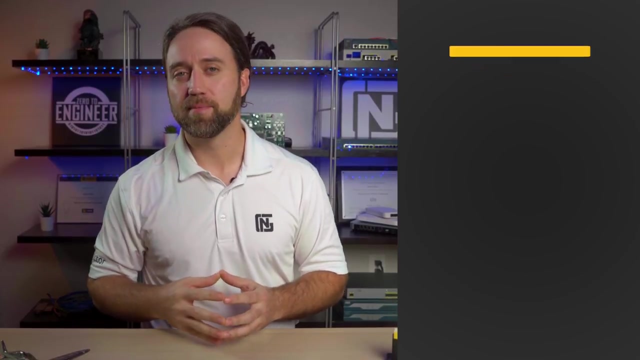 Now the work leads to my number two reason to recommend this career for anyone, And that is job satisfaction. From the variety of work that you get and from helping people fix their problems and from deploying projects, you get so much job satisfaction And after you've been in the career, 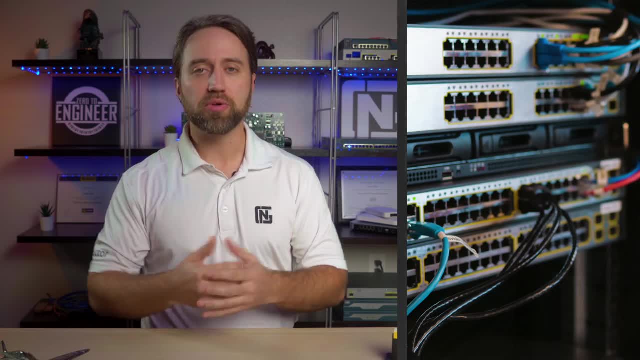 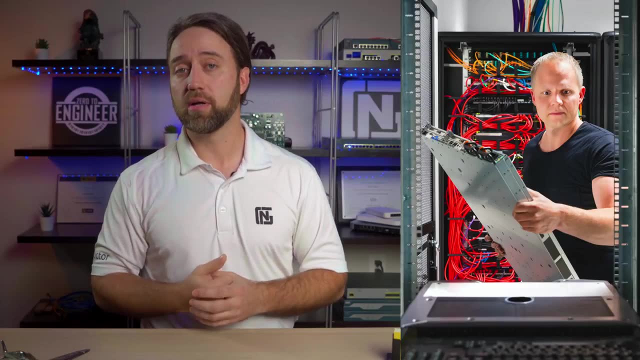 for a little while you get so much job satisfaction. And after you've been in the career for a little while, you get so much job satisfaction And after you've been in the career for a little while, you get very skilled And you get to be the hero, You get to save the day, You get to fix people's problems. There's just so much job satisfaction and fulfillment that I get from the job being a network engineer that I would literally recommend it to anyone because of that. So that's my number two. 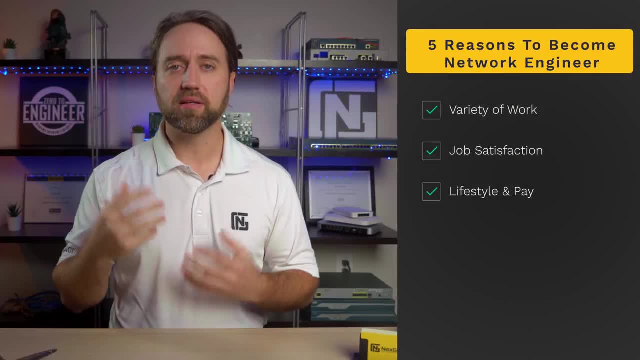 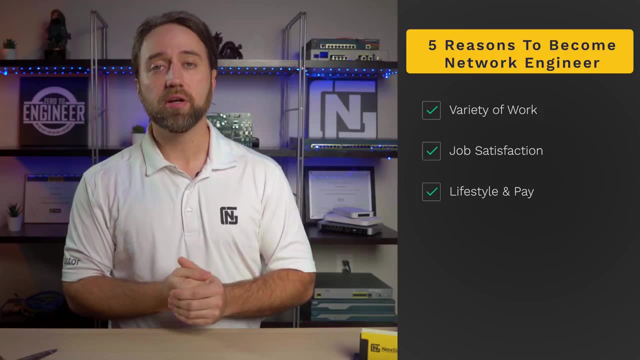 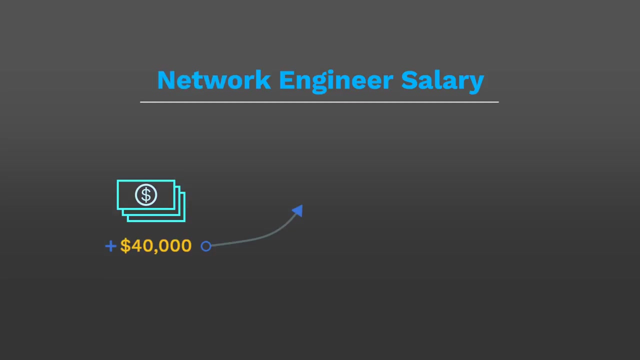 My number three is now actually the lifestyle and pay. Of course, the pay is good. It's a great side effect, And what's great about the pay as a network engineer is it can range vastly. Starting out it could be as low as $40,000, but I actually have friends who are in networking making over $250,000 just doing networking. $250,000 per year- Now that's on the high end, of course, but you can find yourself anywhere in between And achieving a six-figure salary is very, very, very important. 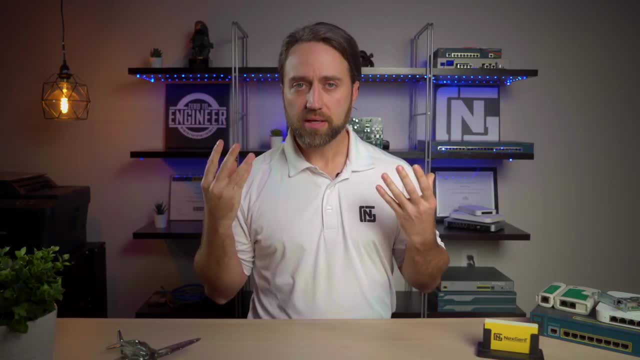 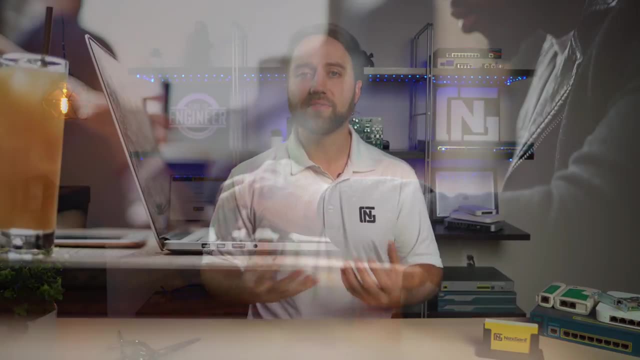 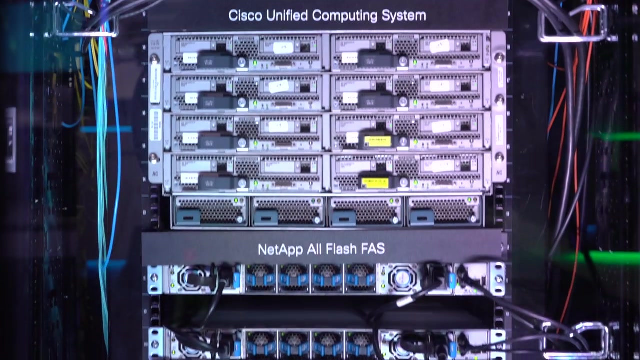 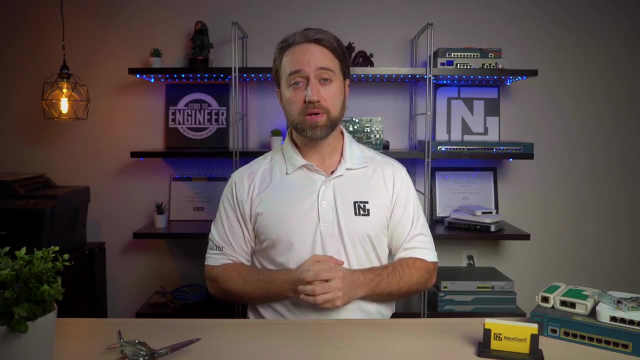 Now, it's the pay, but it's also the lifestyle here that I'm associating together as my number three, because you can also create kind of any lifestyle you want out of this. You can be working remotely or you can be having a mix of working remotely and also on site. So the lifestyle and the pay and things that come along with that, that's my number three, My third reason why I would recommend networking as a career for anyone. And my fourth reason is the flexibility, This kind of association with the pay. 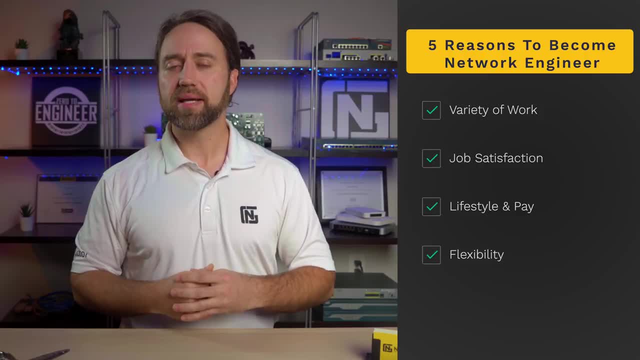 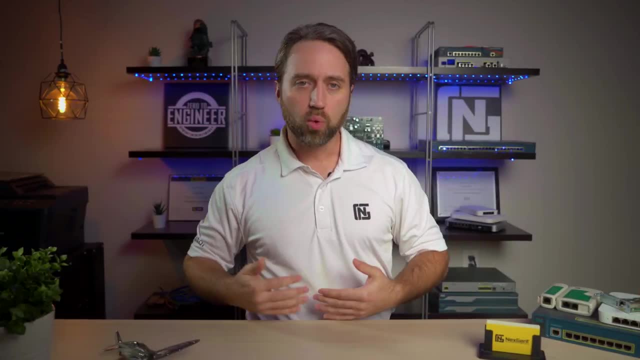 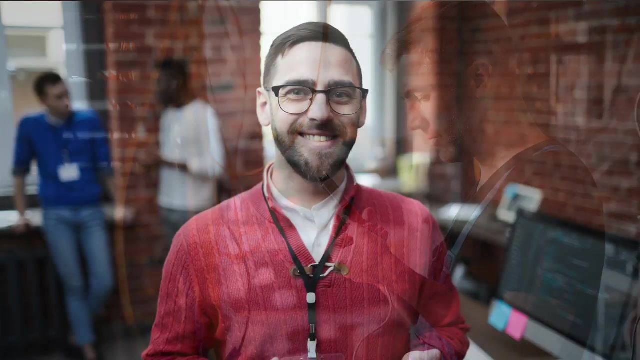 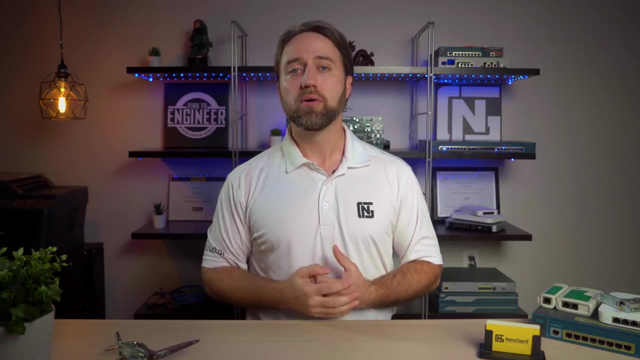 I don't just mean the flexibility that it gives you to work from home and things like that. I mean the flexibility of the job itself. You get to be indoors and outdoors, You get to have a dynamic environment. You can be in data centers or in front of people, You can be in your office or out in the field working on a job site. There's just so much flexibility to what the job entails that it adds to well the enjoyment of the job itself. So that's my number four And my fifth and final reason why I would recommend networking as a career for anyone. 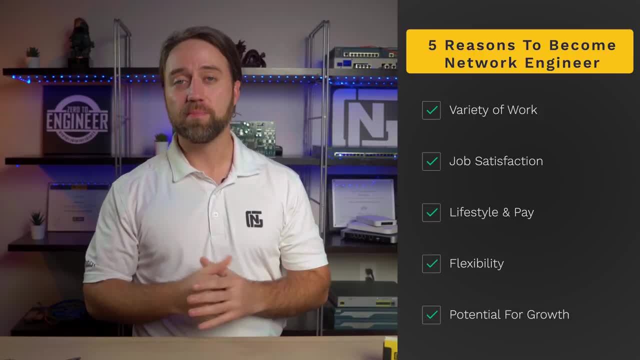 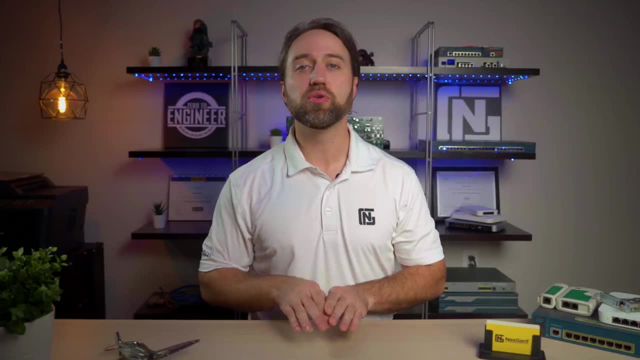 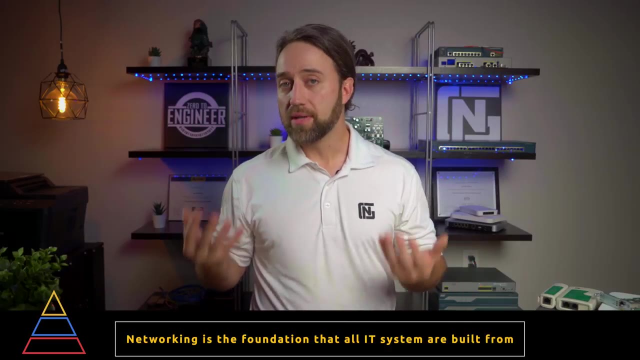 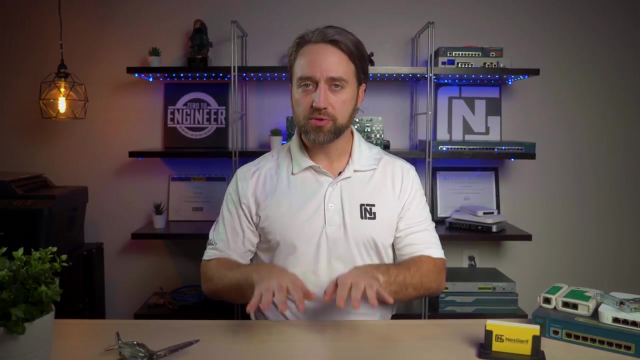 I would recommend the network engineering career field to anyone is the potential for growth. Getting into networking is like planting the best seed that you can if you're trying to get into an IT career. Understanding networking is the foundation of what all IT systems are built from, So networking knowledge will actually help you in any career path that you want to get Now. I don't just mean the potential for growth into other career fields, although you can move into like wireless networking. 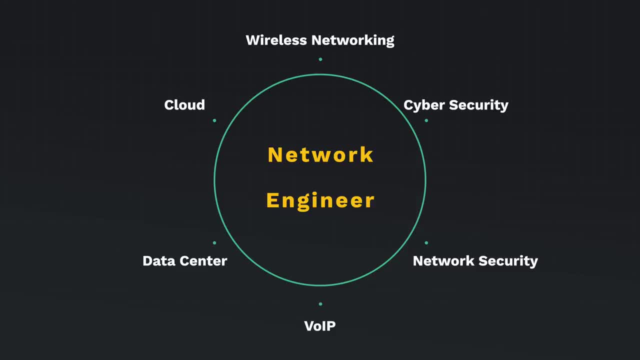 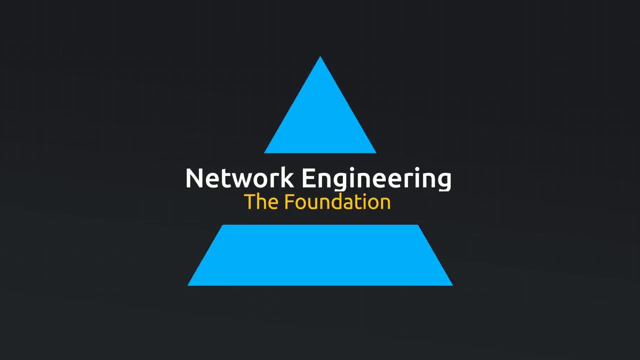 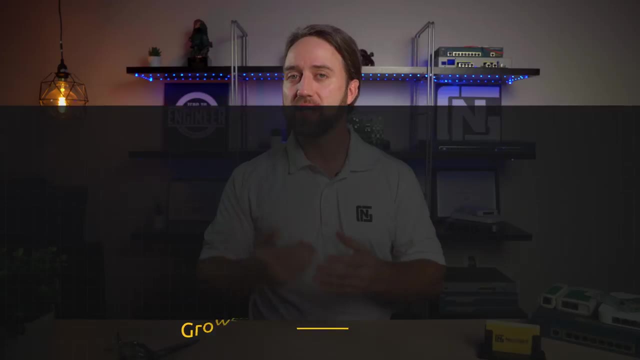 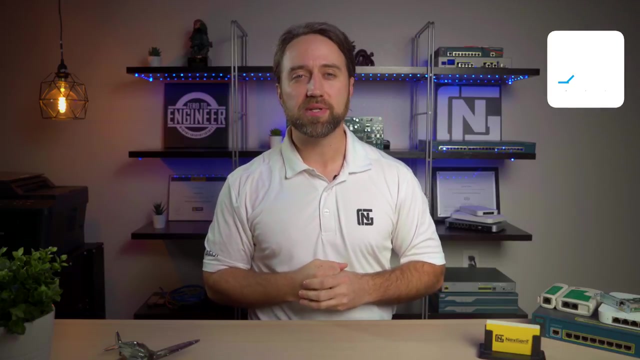 cybersecurity, network security, voice over IP, working in data center, working in cloud. There's so many different areas that network engineering as a foundation can lead to and help you grow into, But you can also grow as a network engineer itself, And that's what I did in my career, And I would recommend that to anyone as well. So that's why my fifth reason for recommending the network engineering career field is its potential for growth, Because it's got more potential for growth, I think, than any other starting point in your career. 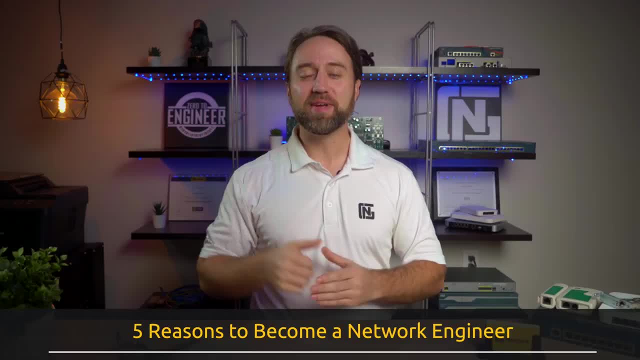 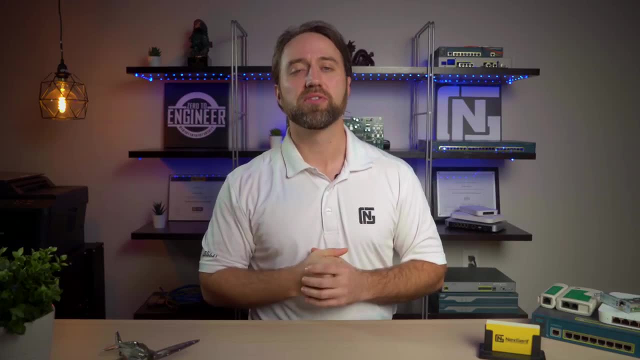 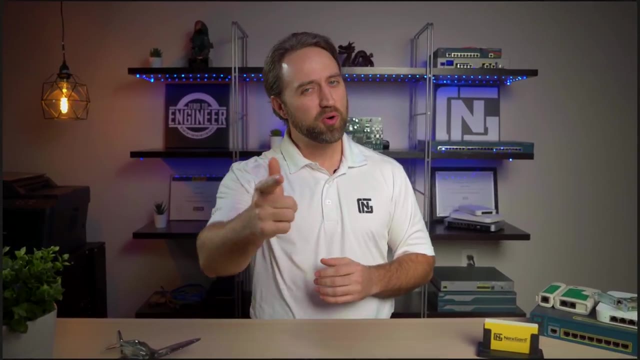 All right. well, those are my five reasons that I would recommend the network engineering career field literally to anyone, And I literally think that anyone can do this job. All right, folks. Well, if you like this video, please like and subscribe. This is Jacob Hess, your instructor and mentor, and I'll see you in the next video. 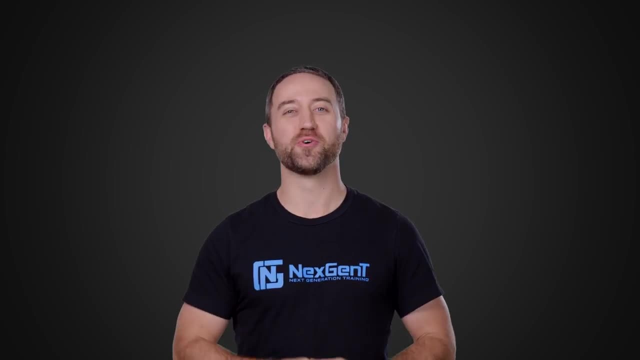 Jacob Hess here. Thank you for watching the video. I hope you really enjoyed it, And I'd also like to remind you: if you're truly serious about your career and information technology, be sure to check out our IT engineer training programs at wwwzerotoengineercom.